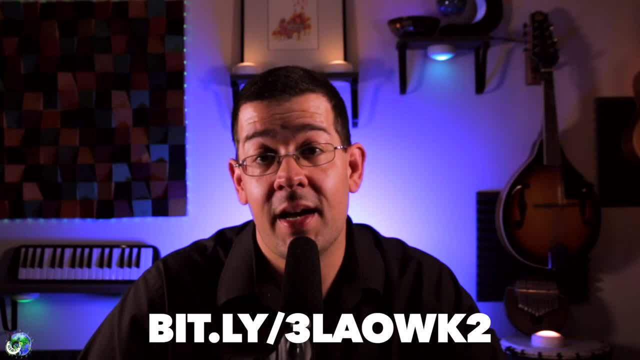 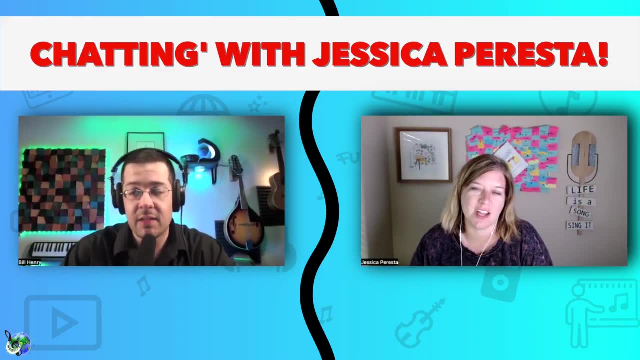 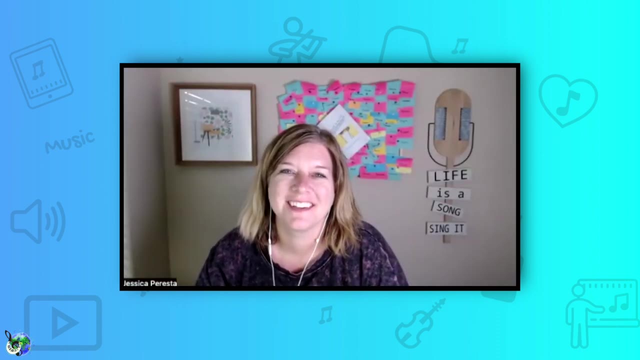 coaching week, or follow the link in the description box as well, but let's dive into more of what we see during the week with Jessica. Jessica, and welcome to the channel. thank you so much for having me- absolutely so. thanks so much for being here with me, and today we're going to get some. 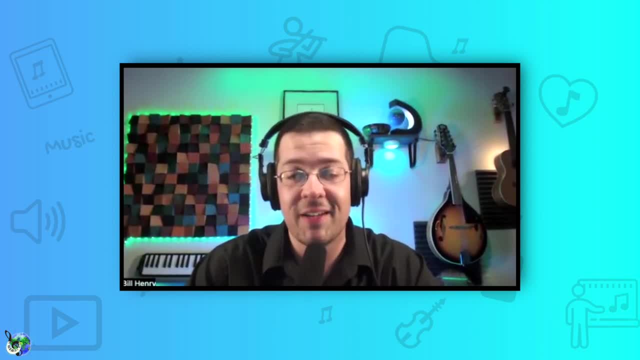 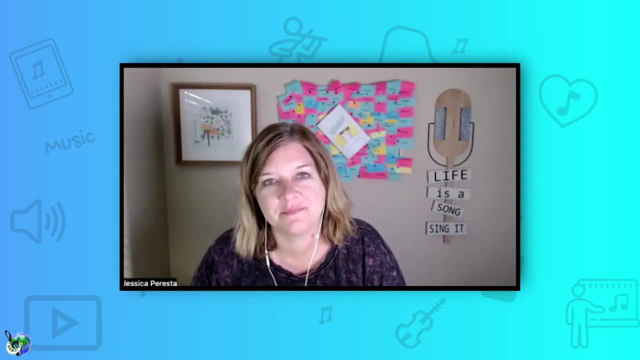 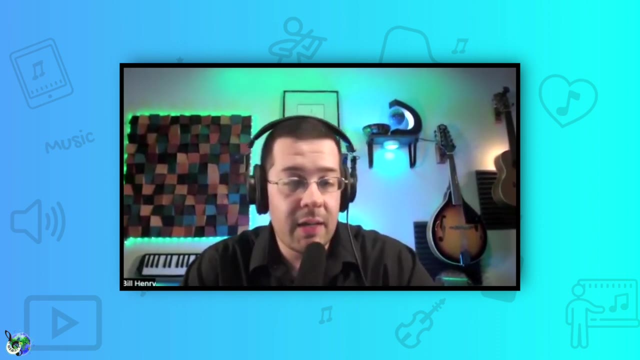 insight into a free week long elementary music coaching extravaganza. that's what I'm calling it, the extravaganza- and it is free- which is really going to give teachers some push for the start of the next year. And you know, personally I know that if I put a little time aside now to plan, I'm probably going to 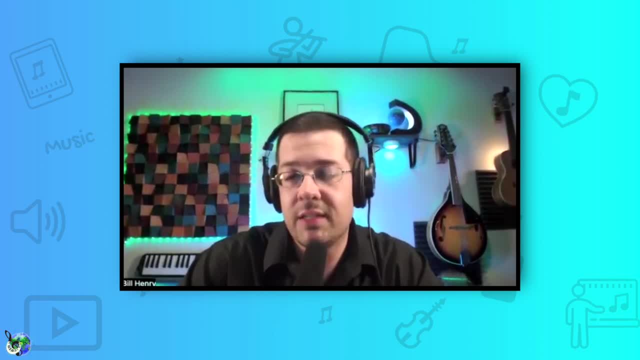 thank myself later. so I'm just really interested in today's discussion of learning a few strategies that will be emphasized during the daily sessions during the the week coaching, one being how to simplify lesson planning and also discussing mindset. then learning more about what's involved during the week of the free coaching. 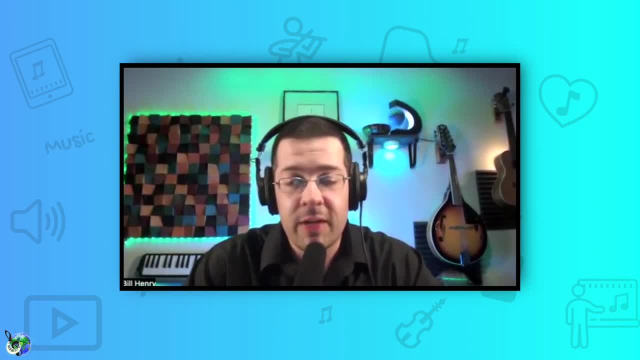 But before we get to that, I want to just say thank you so much for joining us today and I hope you'll have a great day and I'll see you next week. Thank you so much. It would be great to just learn. you know more about you, so could you give us some background about? 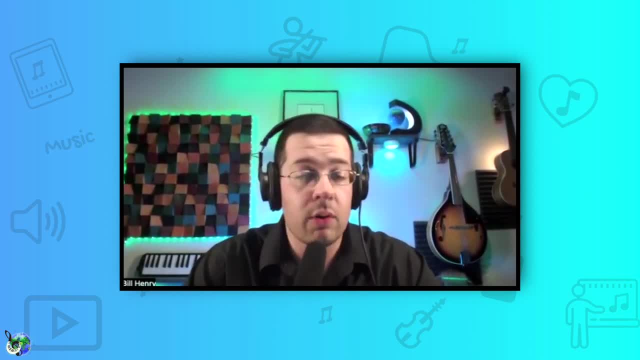 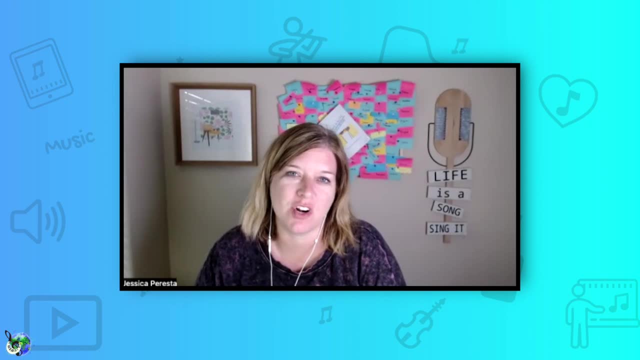 yourself your music teaching journey and where you are today professionally, Sure. so I graduated with my bachelor's in music education in 2004 and taught in Tulsa for seven years, and I was one of the weird people that graduated in December and then was just going to. 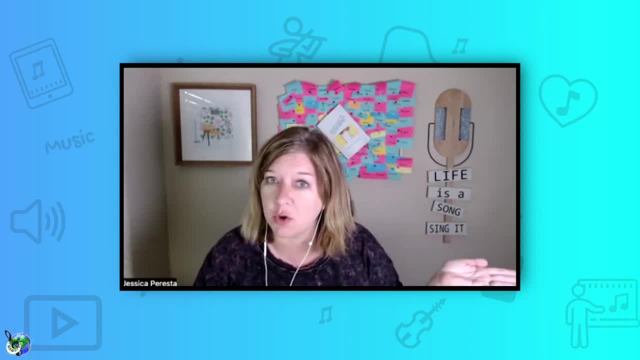 substitute teach and get a teaching job that fall well. one position opened up In Tulsa public schools and I got the job. so didn't know at the time, though, that the school had had a music program for seven years and no instruments, had no curriculum, had nothing, literally. wow, and I. 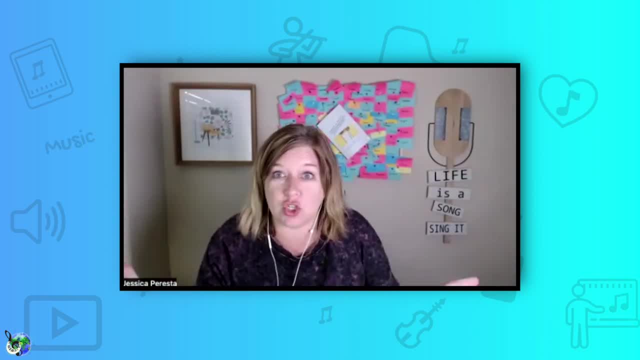 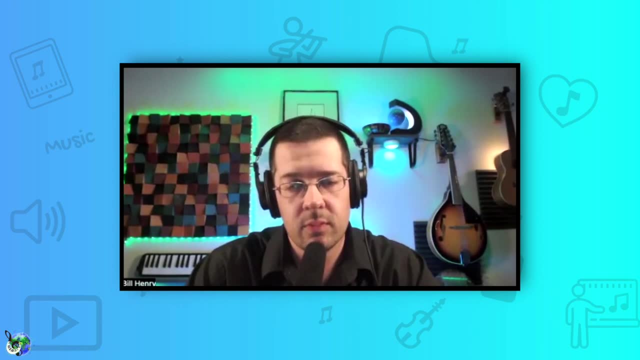 had no budget so I just like it's a job, great sure for out of college. so, lo and behold, I took the position he had. to make a long story short, I built the music program up once they're actually seven years, so seven, some magic number apparently in my life. and then 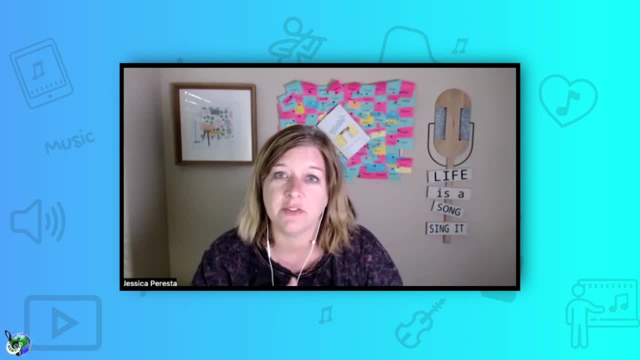 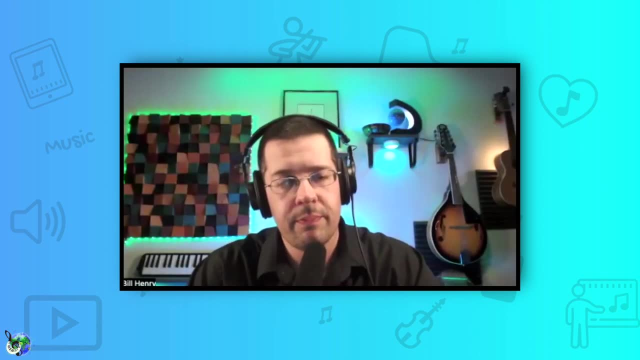 We, my family, moved to Arkansas, transferred my teaching certificate with every single intention in the world of going back into the classroom, getting a job here. yeah, and I was pregnant with my second son and then we had a third boy. we found out our oldest had autism and our middle 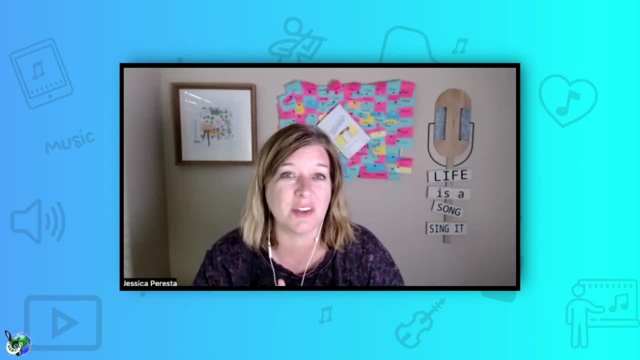 son had seven food allergies and I did not feel comfortable putting either of them in daycare. so, yeah, I said okay, I don't know for how long and I don't know how we're going to make this work, but we're going to make it work and then I'm going to go back to the classroom. well, 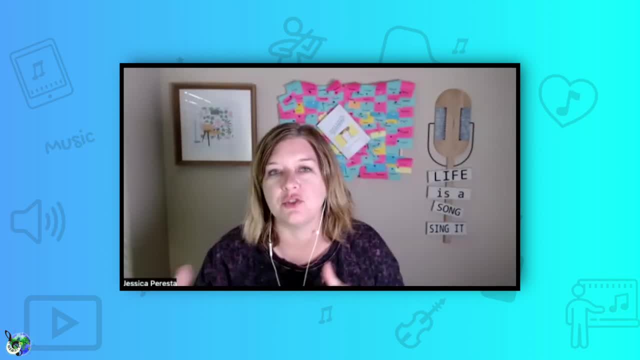 when I kept. when I was in the classroom, I kept getting asked the same questions by teachers at PD or wherever. if they would hear my story, they're like: well, how did you do that? how did you teach without a curriculum? how did you teach without instruments? how did you? how did you? how? 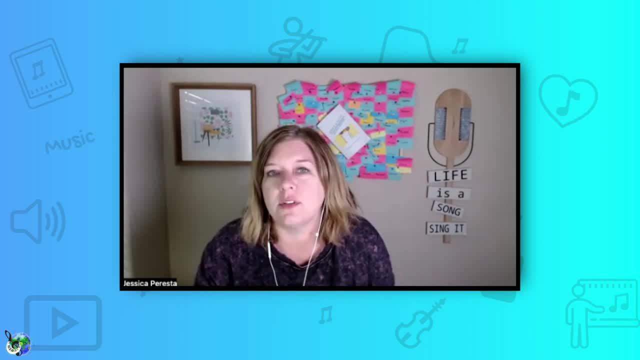 did you? and I was like sure, I just kind of figured it out. and then that's the honest truth and I finally was like, well, maybe there's something to that, because I love mentoring teachers. I loved, I loved having student teachers. so I thought what could I do with this while I'm home? 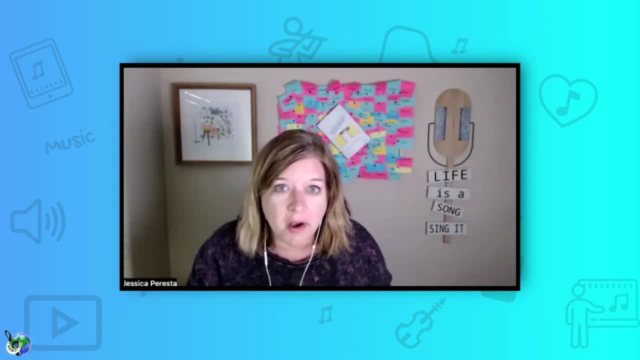 I go back into the classroom. what could I do to help? so I started a blog. it makes it sound so easy. I just started a blog. no, it was not that easy, trust me. my husband, luckily, is very techy and helped me build a website and all that. but anyways, it just started with. that turned into a podcast. 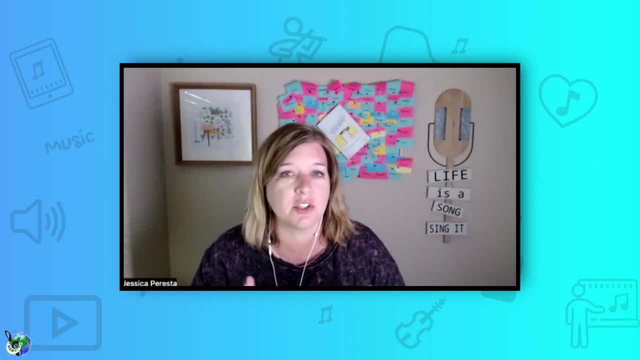 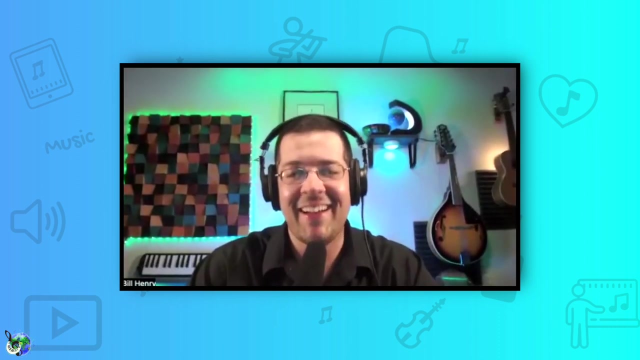 the elementary music teacher podcast turned into a book, turned into a membership site and just grew, and naturally so I am doing this now full-time. never in a million years did I think this would be my life. and seven years later, here I am still. it's really seven years right? yeah, I know, I'm telling you seven is the number. well, I think. 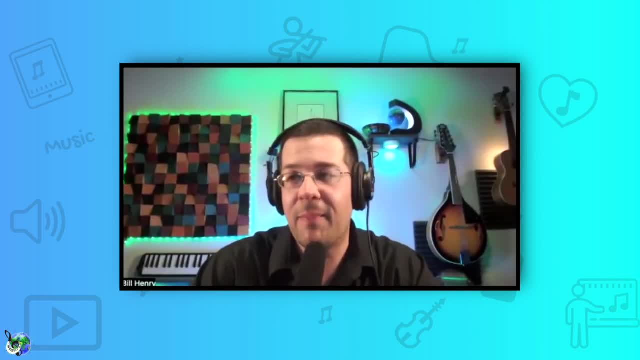 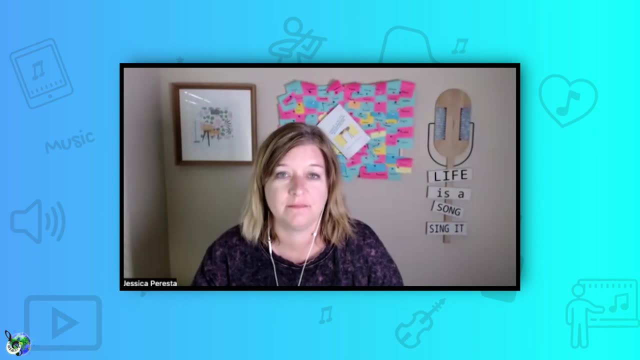 you're right about that. I think five to seven years. you know, yeah, my mom was a music teacher and she said, yeah, it's gonna take you probably five years to build the program at your school. yeah and yeah. so I think, yeah, that's definitely a thing. so, but sorry, go ahead and continue. no, 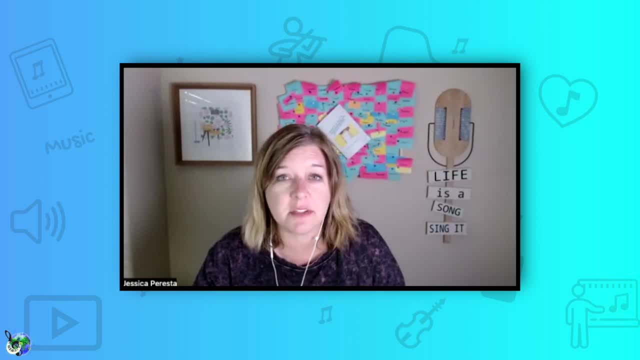 so that's, that's what I'm doing now. I am now running my business full-time, where now I get to help music teachers be your best selves in your classroom, and I love it. so, yeah, that's where I'm at: to help music teachers be your best selves in your classroom, and I love it. so, yeah, that's where I'm at. 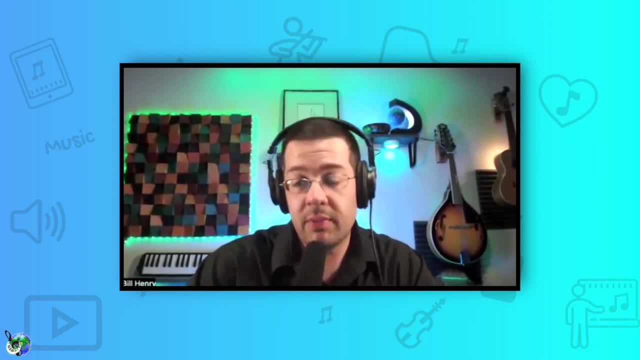 that's so great, so one of the sessions- aware that I am so great, so one of the sessions- to help music teachers be your best selves in your classroom, and I love it. so, yeah, that's where I am discuss is simplifying your lesson planning to help music teachers be your best selves in your classroom. 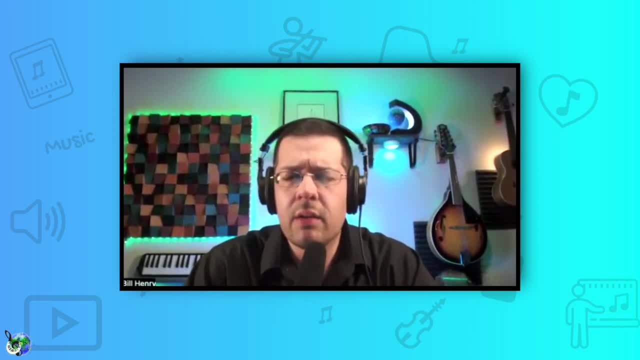 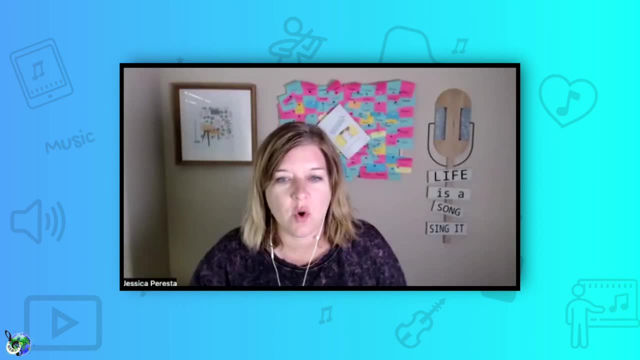 um, and you know there will be more within. discuss is simplifying your lesson planning that session. but tell us a little how we start the. our coach and that's watches learn a little right of a tortured. better plan something to lAdd some story you read of a visual. 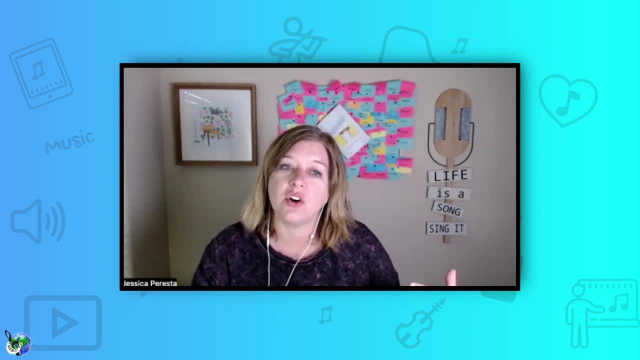 experience that interests and feel the, the social connection. but I am so criticized I do enjoy it. just because I love it so much, I must like it when it's interesting, it just rather. I won't miss my class and I waste my drei. so glad, looking back now, i started with nothing, really, because i was able to build out my own. 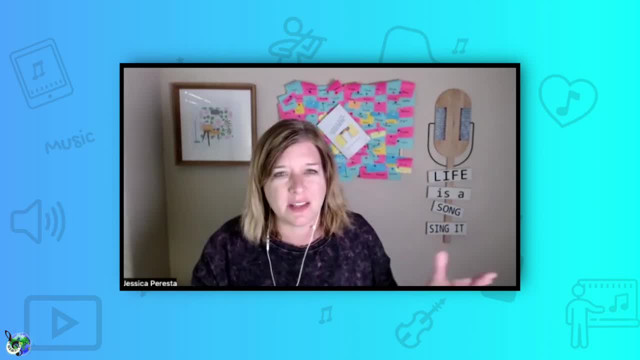 curriculum um, slowly get the resources and lessons i wanted, and so i think for most teachers, when i was thinking about this question, the overwhelm comes from either having not enough resources, like i was in, or having too many, or not having a scope and sequence or curriculum map, or having too 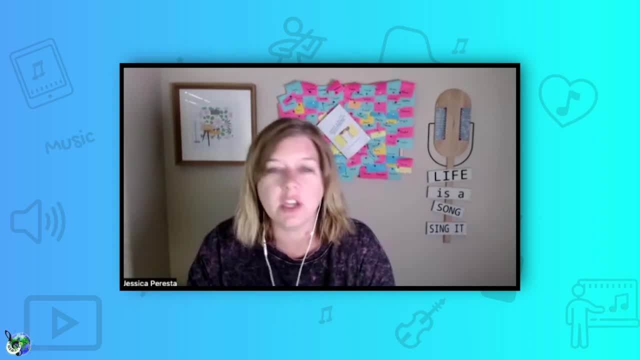 many, because a lot of times when you, you know, subscribe to an online curriculum or you have in-person curriculum, it usually comes with a curriculum map. so then you're left with like 10 of them and you're like they're all similar but a little different, and it's overwhelming. 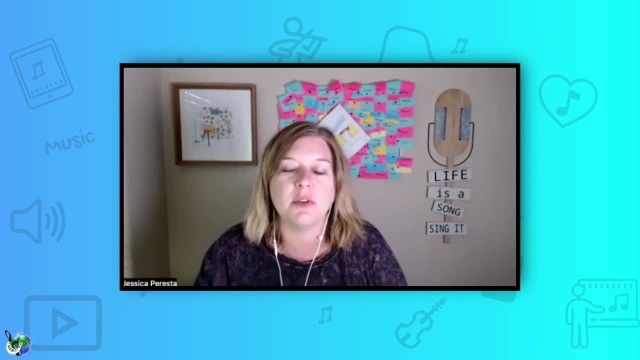 um, and so those things will cause the overwhelm. so, when it comes to simplifying lesson planning, what really has worked for me- and i'm getting my master's in educational technology and we really talked about backwards planning a lot and i never put a name to what it is- 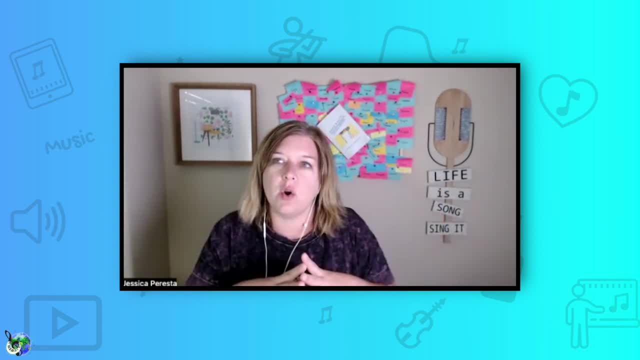 but this is what i did. you start with a bigger picture where not- and some people just do this, but i know some music teachers do not- right where. what i mean is you look at the full year and then you break it down by nine weeks. and then you break those nine weeks down by weeks and focusing on the 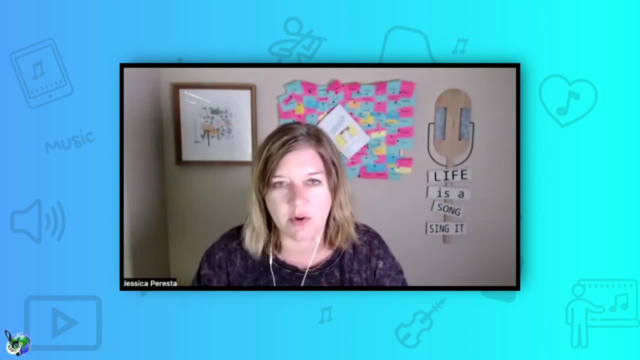 grade level. so it's about- and we're going to cover this in a lot more detail- but the main things about simplifying lesson planning is staying organized using the resources you already have available. first, but right, you have things already there, even if it's just one lesson. 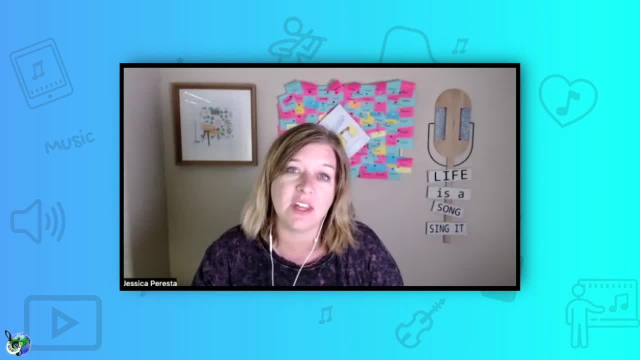 right um having a running list of songs and activities that you can teach to the concepts, because focusing on the concepts before looking for the songs, which sometimes those things are reversed, knowing how long you see your students is huge, and this will um help you with knowing how much to fit into a lesson plan. and then the last thing i say when it comes to simplifying: 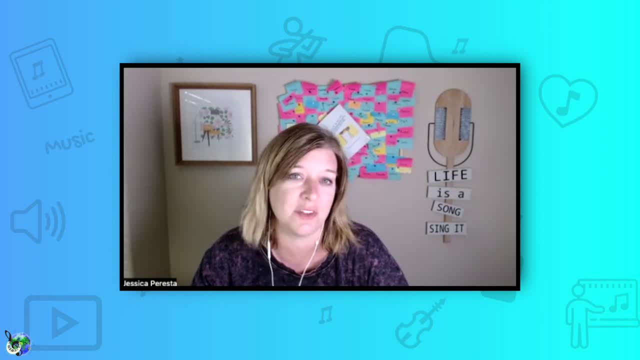 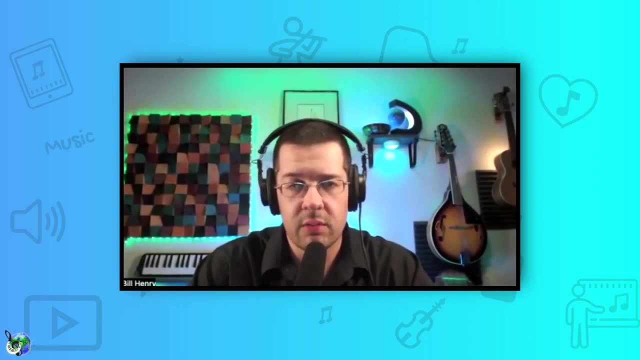 lesson planning is to stay flexible and know that no two classes learn the same way, and that's okay. so we will cover all that a lot more. but yeah, yeah, that's cool and i love that idea of really just looking at the big picture first and then getting because you 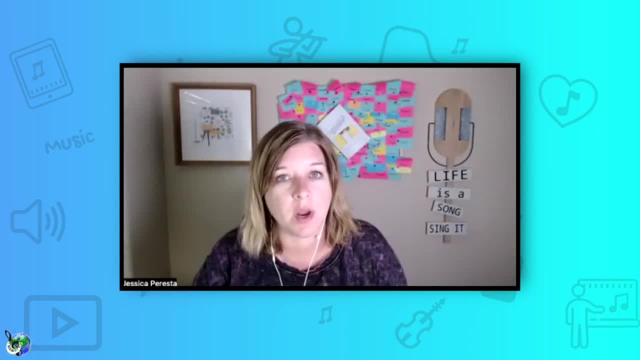 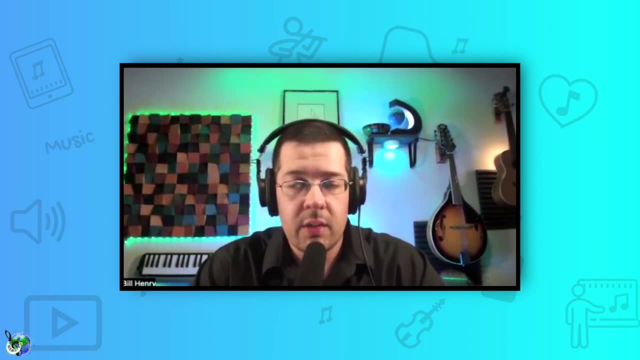 it's just, it's easier to manage, right, because it can just be a lot if you're just looking at one little specific thing. so, yeah, right, yeah, that's great. so another session during the week is to discuss mindset. uh, so tell us more about what to expect, like, in regards to mindset, like 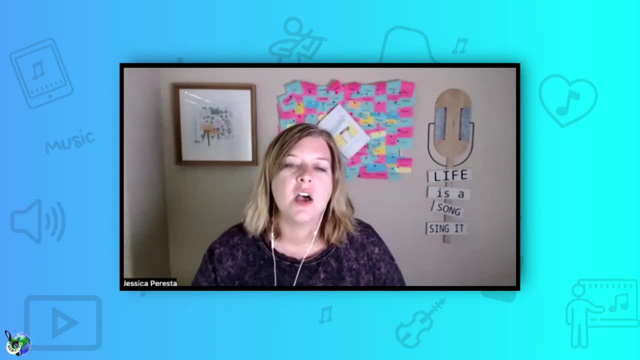 what exactly do you mean by that? like, what does that mean? yeah, yeah, so when i was in the classroom, i actually wrote a book, and that's- and this is not to me- plugging my book. but the reason i wrote my book was because of the things you don't really know until you get in the classroom. 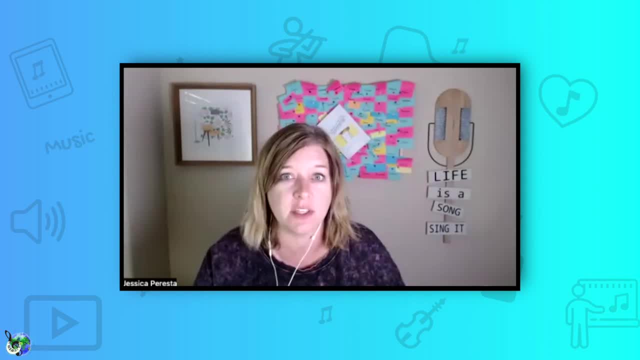 you're just told: teach music, but there is so much more that goes into being a music teacher than just teaching music, and i don't mean just teaching music, but you know what i mean? yeah, there's. so there's definitely mindset struggles music teachers face day in and day out. 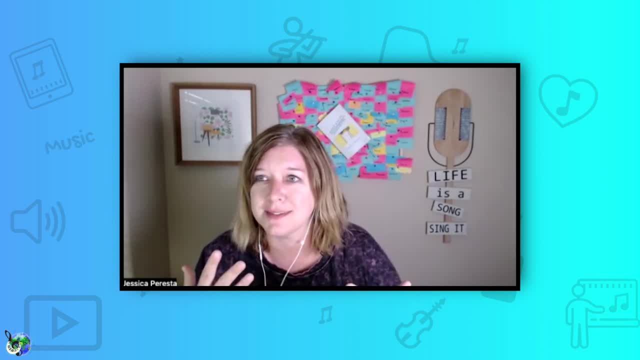 and, like i said, a lot of it has to do with things outside of teaching music and, a lot of times, two or three different things that i've been able to do with my mentor. i see them comparing themselves to what others are doing based on what they see on social media. but that's the highlight reels and 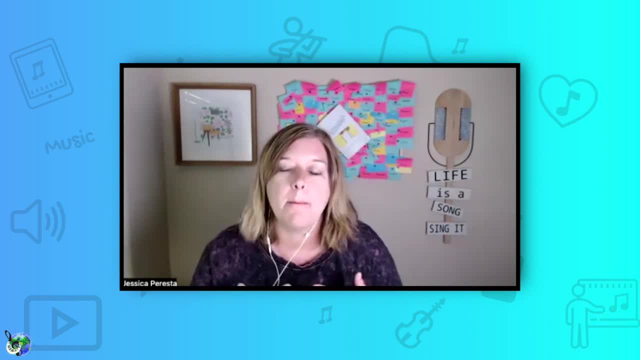 it's that, that's the good and that's great, like we want people to experience good, sure, but i don't feel like a lot of times what's talked about is the hard. is that i'm struggling with this. this is hard and um so during coaching week i there's a lot that goes into mindset. it can be a lot of. 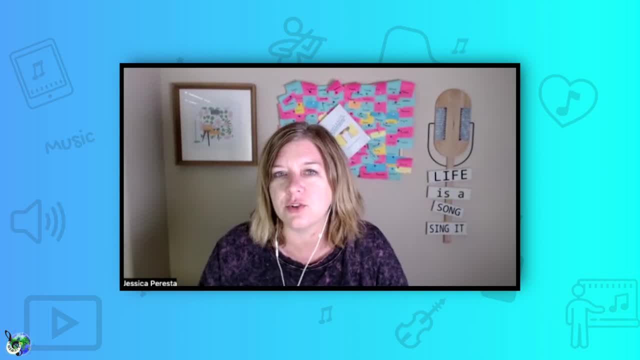 different areas, but we're going to focus on three main areas and there will be some question prompts during the week and then the facebook live will just kind of address all these areas. one is about work-life balance, um, which that can be a million different, you know, go a million. 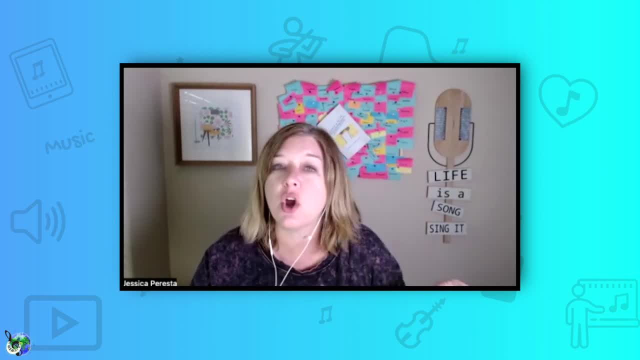 different ways too. another one is about getting ready to go back to school. there's so many mindset things you're thinking about and dealing with when you just think about that topic alone and then the ins and outs of teaching elementary music, your mindset around that like what i mean. 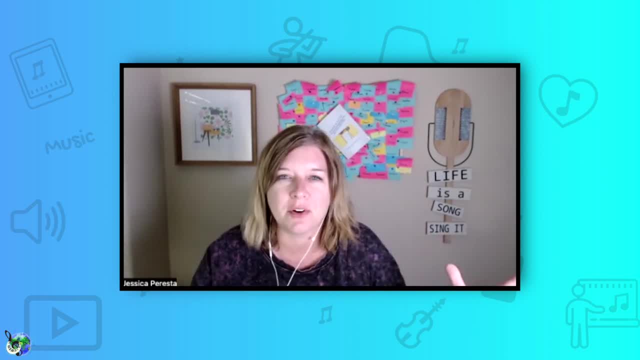 you just got a lot of feelings and, uh, maybe it's certain people or colleagues that made you feel a way, or maybe you used to love your job and now you just have kind of lost that passion and we're going to just kind of touch on some of those areas and help you move forward in getting hopefully. 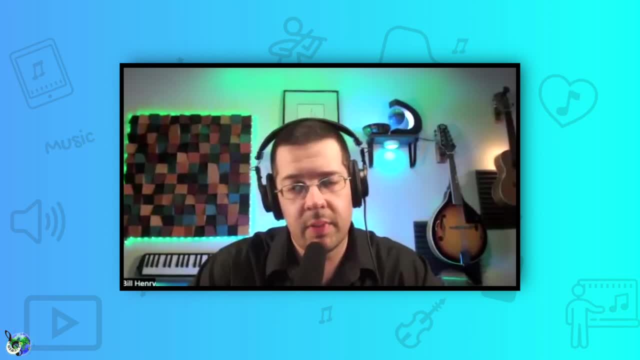 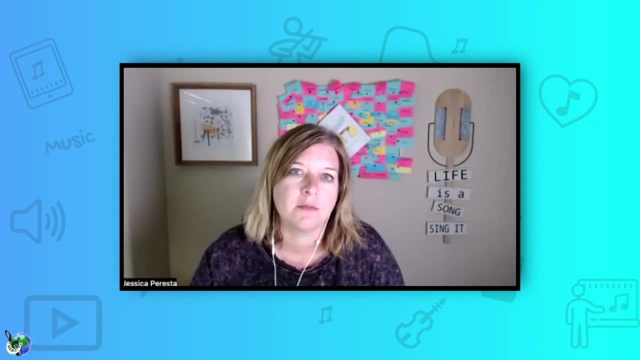 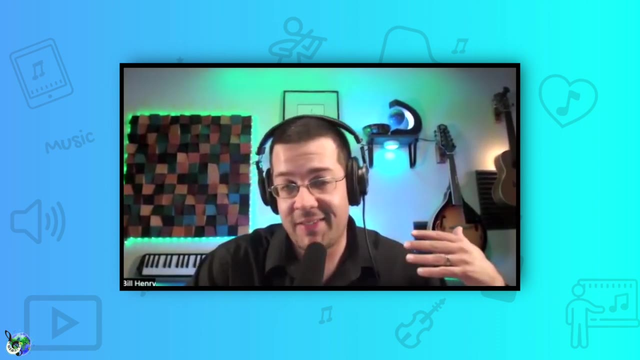 past them a little bit, if you can. yeah, that's awesome because, yeah, you're right, there's so many different aspects to it. you're not just in there teaching, um, you know, i think sometimes, like when people perform, like the best part of performing is getting up on stage and doing the performance. but 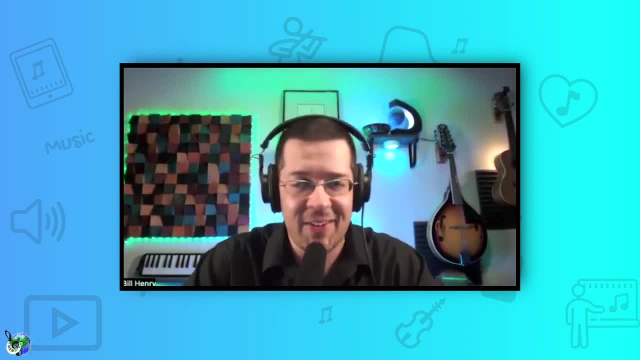 yeah, then you got to do it. you got to get up on stage and do the performance, but then you got to tear everything down, right, that's like all the, all the stuff that you don't like. yeah, you don't even like. think about that, you have to do that, and there are so many layers of that within the within. 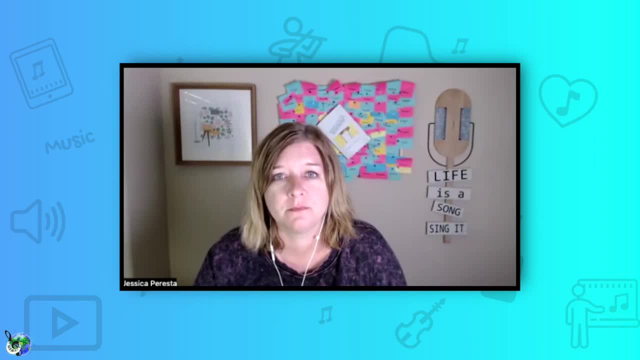 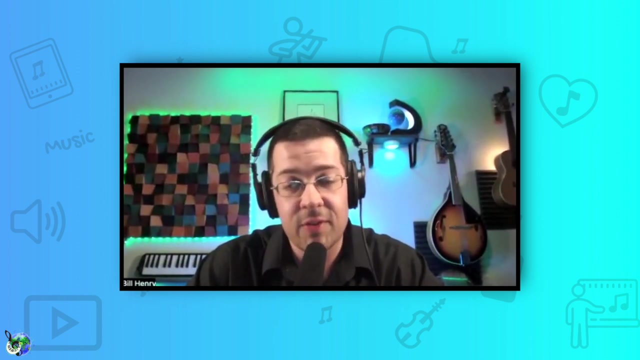 the teaching profession. just in general, yeah, so, and then, especially as the music teacher, you know, there's so many different things that you have to organize and do and are expected to do so, absolutely, i was just going to say. another part of the week is um getting the first month of the school year. 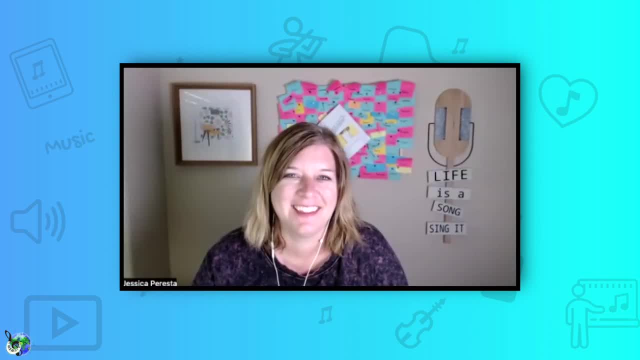 out, which is great. So tell us about how that session will work. Yeah, So I know that's a lofty goal, first of all. So my goal, like I said, is to help you plan out your first month. But what I 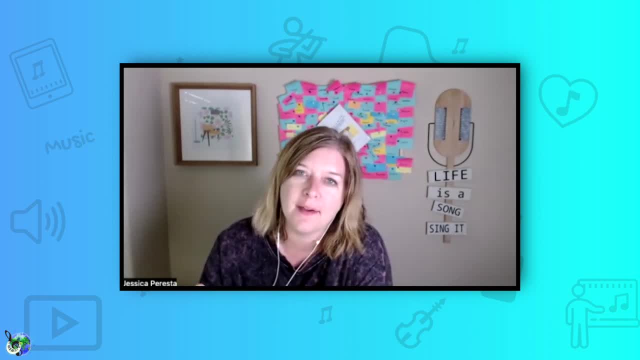 also say is: my goal is to help you be on your way to doing that. So if you leave that session you're like wait a minute, I'm not, I just have one week. That's great, Like we're going to. 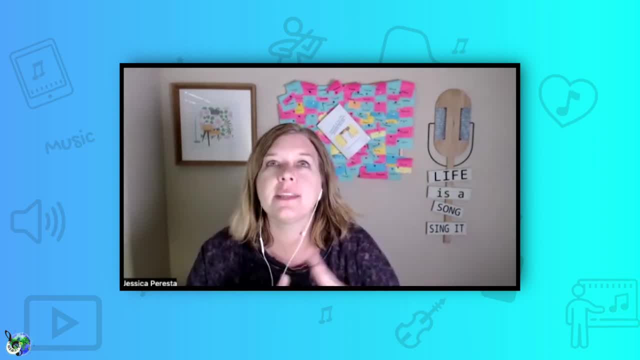 celebrate your wins, no matter how big or small. Yeah, The reason I'm hosting this session is because I don't know if you can. you can probably relate to this bill A lot of times. the elementary music teacher- you're the only one in your school building. I did my student. Yeah, My student. 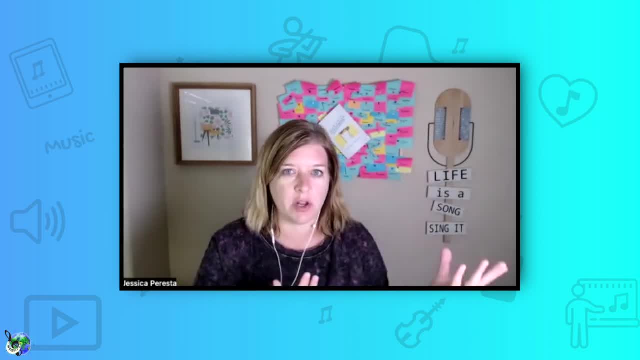 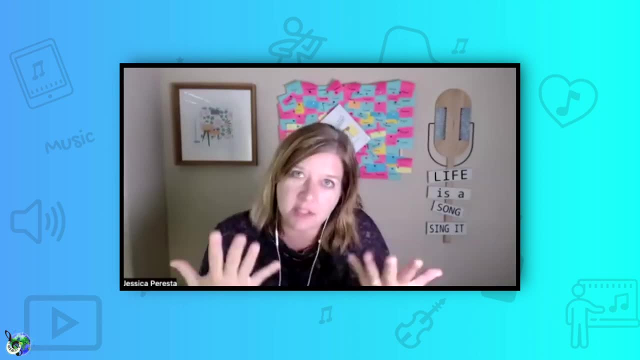 teaching placement, though I don't know a lot of schools like this, but they had a lower elementary music teacher and a higher grade elementary music teacher. Okay, Very rare And I don't see that very often, but, like I said, most of the time though, that's not the way it is. So you see, 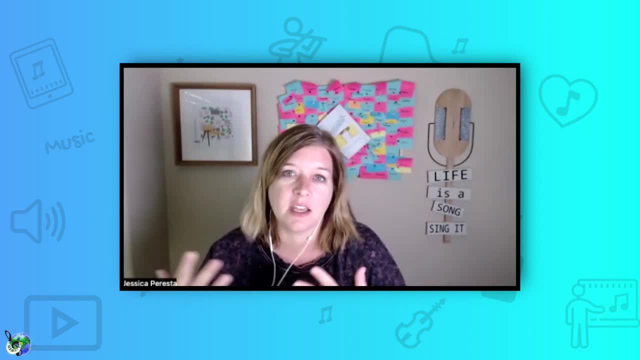 grade level teams planning together in elementary and on secondary you see subject area teachers planning together, But you don't really get that opportunity And you can maybe talk to other music teachers and ask them questions at PDs or or Kodai levels or even online, but it's still not the same as being 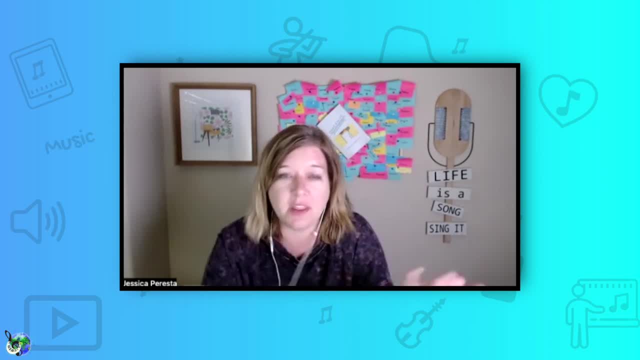 able to come together. It basically is like a like a grade level planning meeting is what I'm trying to put together here, And so this session you'll be able to bring your resources, ask questions, talk about what objectives and concepts you're covering in week one and listen to what. 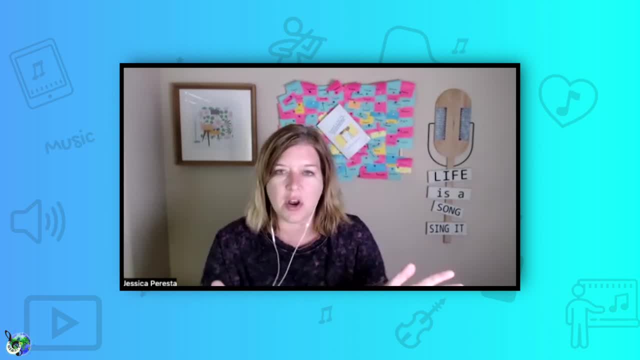 other teachers are doing, So you can. maybe you're not able to sit there and lesson plan, but you can just take notes and be like, Oh my gosh, that's a good idea. So maybe even after the session you're able to go back with 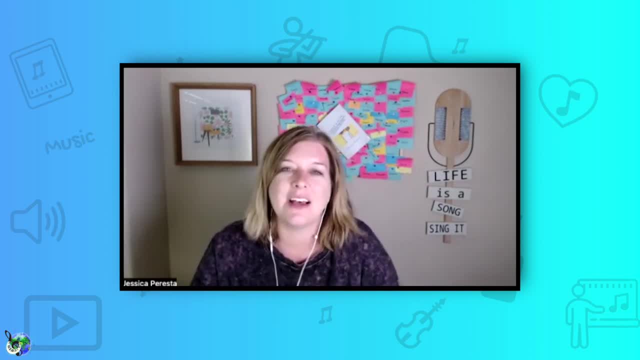 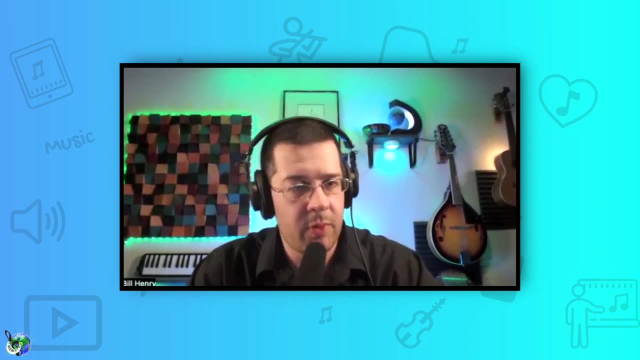 the ideas you wrote down and start planning, And that's the goal. Yeah, that's awesome. And yeah, just to bounce ideas off of others is great And yeah, we do experience that in the beginning of the year with PDs. I feel like lately we haven't had 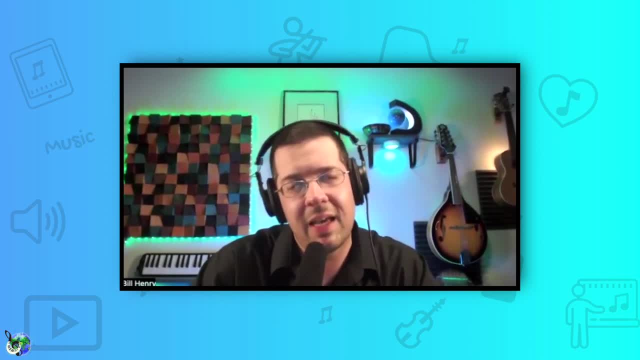 and where I teach in Cecil County, Maryland, we haven't had as many group things together, Uh, but when we do it really is nice to be able to just bounce some ideas off and not only to get ideas from others, but even just to kind of make it like: okay, yeah, I'm doing this, right, Like 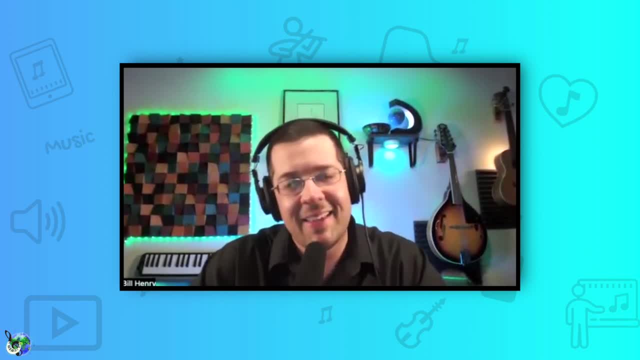 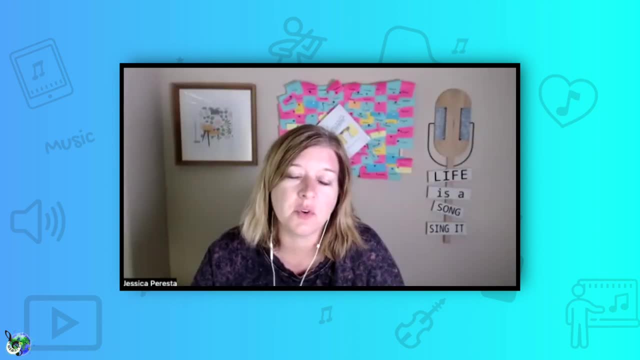 this is. this is what we're supposed to be doing. You know, it just gives you that, that um validation in what you're doing. So I think it's that's really great that you're doing that. So, yeah, Yeah, I'm really excited. It's going to be awesome. Yeah, That'll be fun. So in the intro, 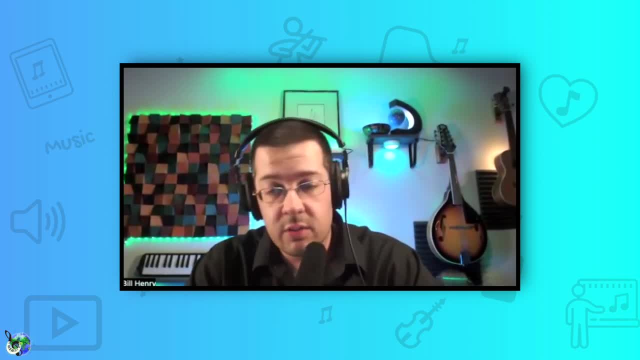 I mentioned that all of the live video sessions will be recorded right. So even if you're not able to attend that day or you're out that week because of vacation, all of that great info is recorded and available for replay. And, of course, questions can be asked and answered during the